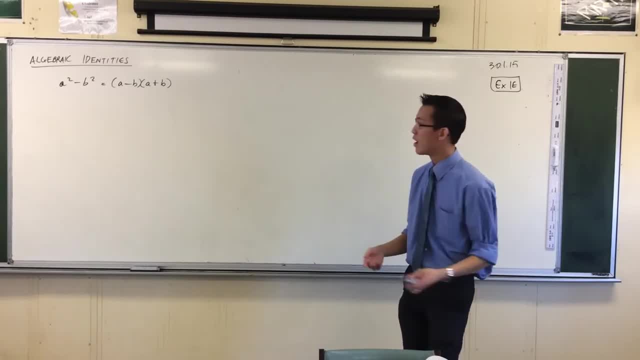 Because some of you will immediately see another way, or some of you might already have been told another way. I want to give the rest of us some thinking time to catch up. Can you think of another relatively easy way to prove it? Doris, your hand went up. 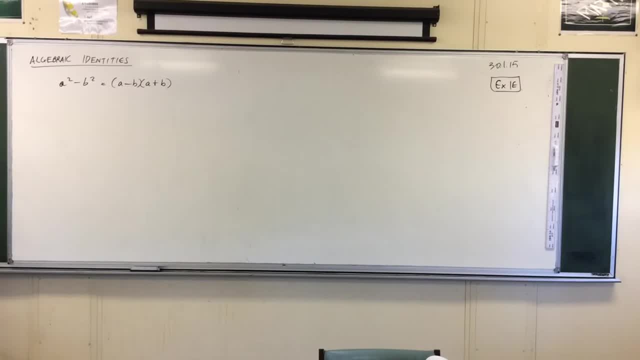 No, I haven't. I retract my offer. Okay, Nikita, what do you think Like rephrase A in terms of B- I don't know- And then sub it in. Is that wrong? There's a couple of different ways to do this. Yeah, Minty. 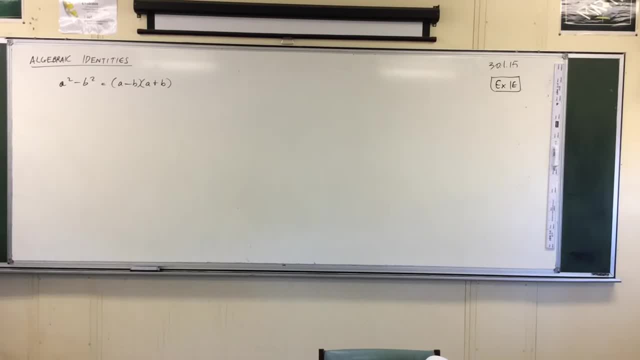 Uh, add A B and Add A B to what Like in the middle You mean here on this side. So I'm going to consider this guy A squared plus A B. Okay, say it again. 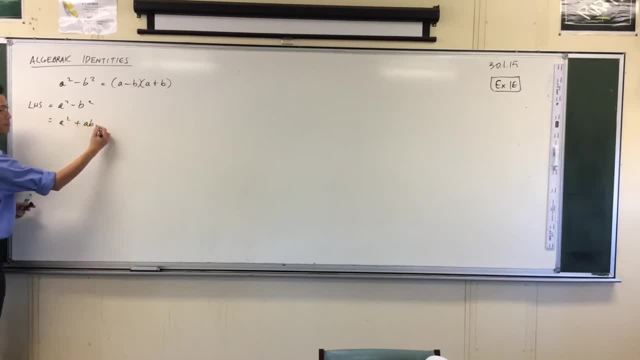 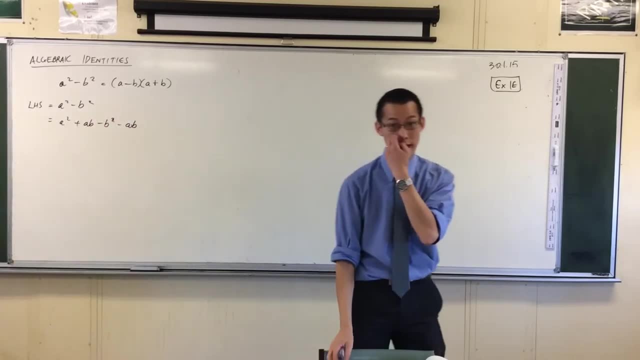 A squared plus A B, minus B squared minus A B. So it's just A squared minus B squared. Okay, see what he did. See what he did. This is a similar thing to completing the square, Isn't it? And actually this is a very important trick when we're learning. 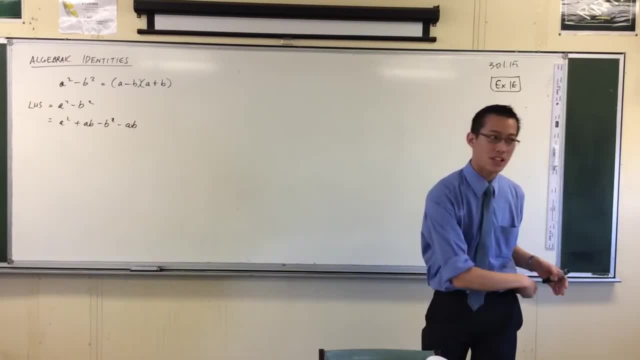 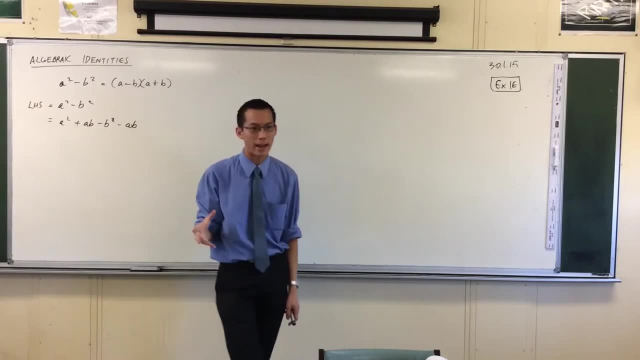 as we will learn a lot more trigonometric identities. One of the main tricks that they pull out of their hat is to say: how do you go from this side to this side? You sometimes have to add something and subtract it straight away. 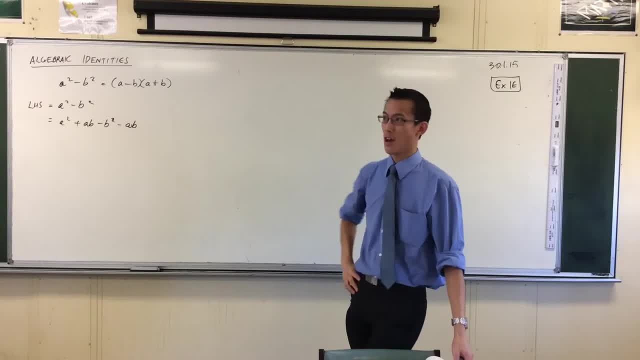 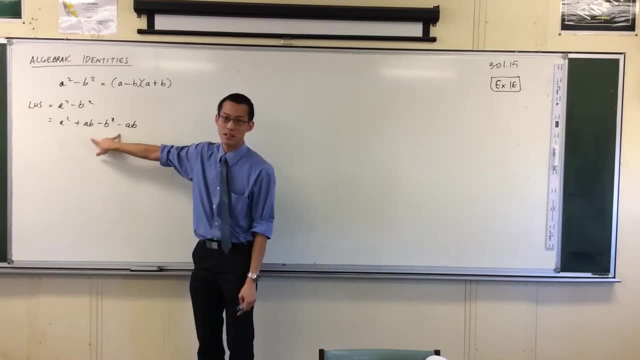 All the way up until like extension. two Harder integration. One of the hardest kinds are recurrence relations, Really really hard calculus And they rely on this simple trick. It's often very hard to see when you're like. you know what should I choose to add and subtract? 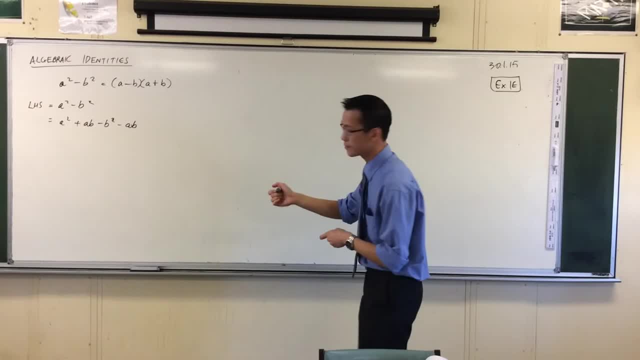 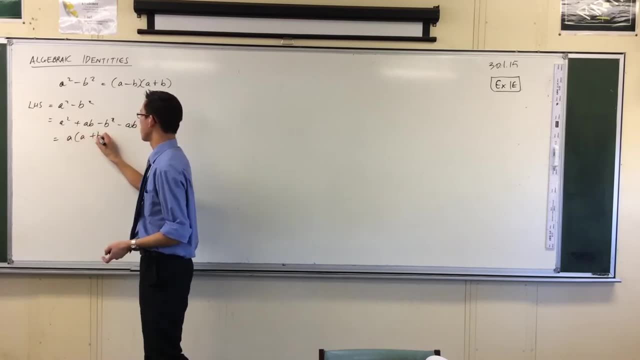 Where are you going to go from here? What are you going to do? Factorize, Okay, now I can factorize, can't I? What should I take out A? I can pair up A from this, so it'll be A plus B. 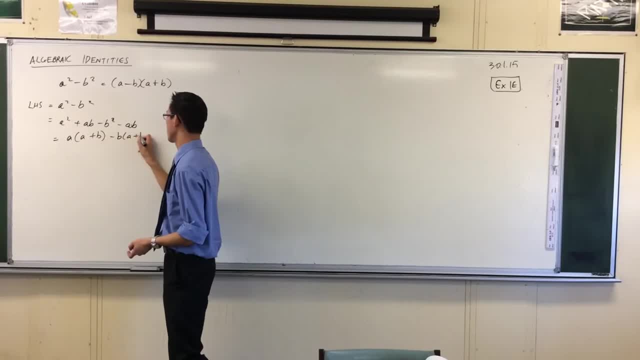 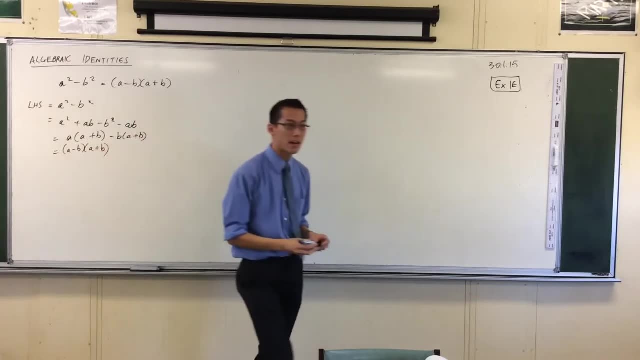 And then Good, And there it is. You can see it now. Excellent. Okay, I'm happy with that. Good, You need to push yourself a little bit. Think about who you are, Don't just settle for one answer. 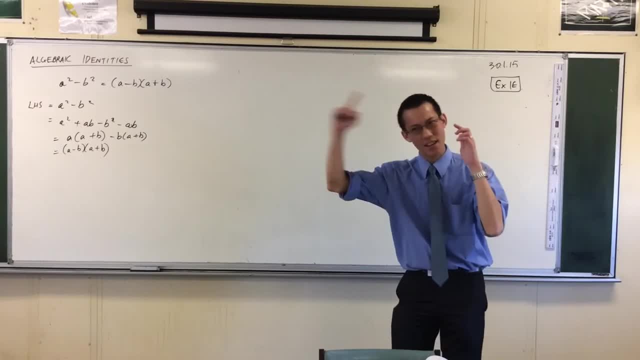 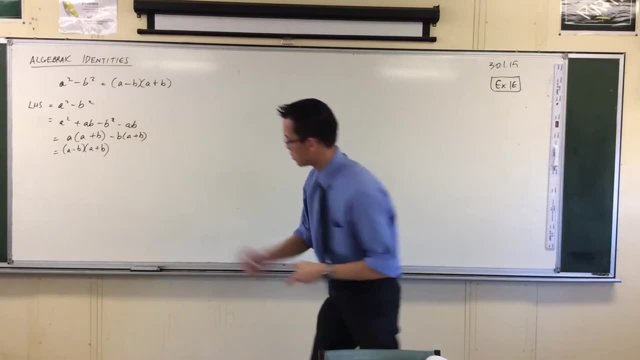 Don't just settle for that way. There's often a way that's not. It takes another route and it might be more profound, more insightful. Let me give you one more, because it's one of my favorites: Which color should I use? 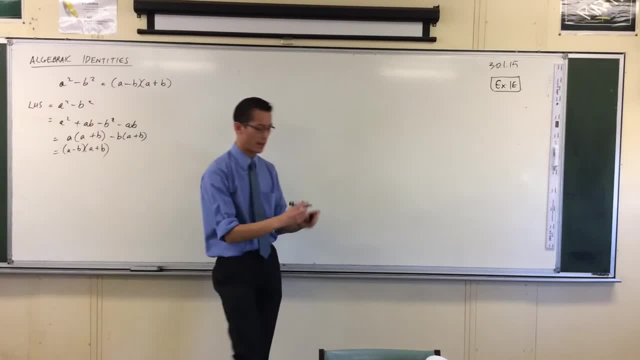 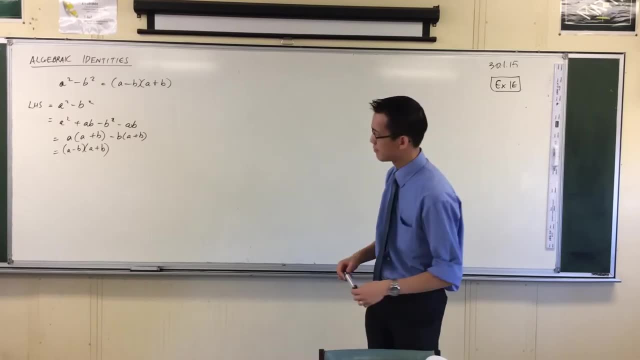 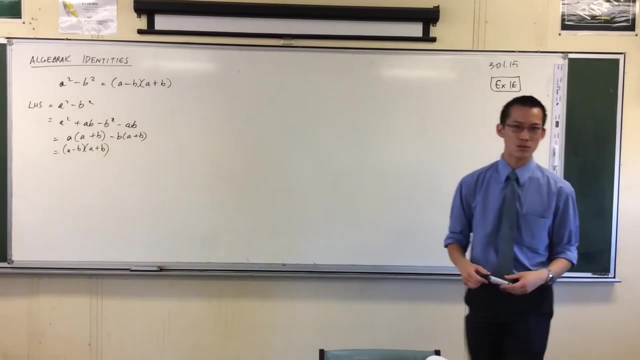 I'll just do this: A squared minus B squared. Why do we call it squared? Why don't we say to the power 2?? Because that's what it is. Why is it squaring And why is it cubing? And why doesn't to the power of 4 have a special name? 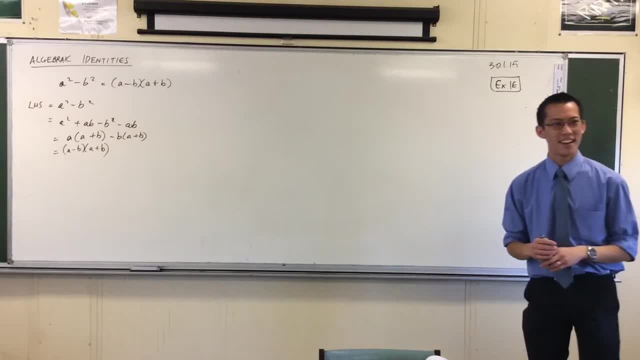 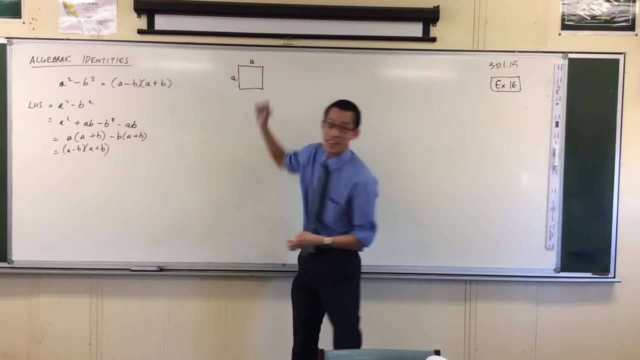 Actually it should. Yeah, Because if you try to find the area of a square, you can't find it. So if I gave you a square of side length, A right, Then its area would be A squared, Because it's a square. 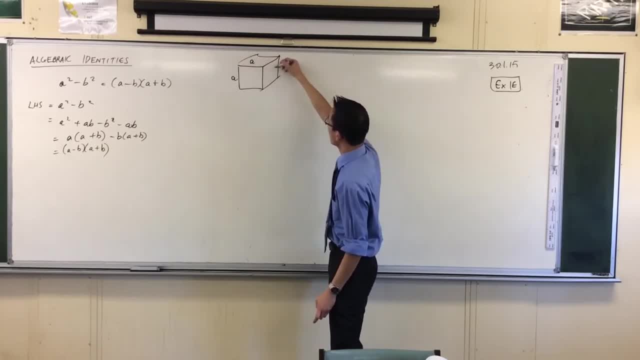 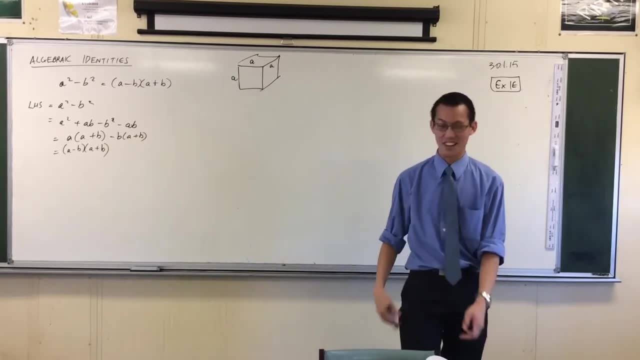 And if you went three dimensions, it's A. Which one do I want? Cubed, Because it's cubed, And if I went four dimensions, I guess it would be A Tesseracted. I don't know. That's a four-dimensional cube. 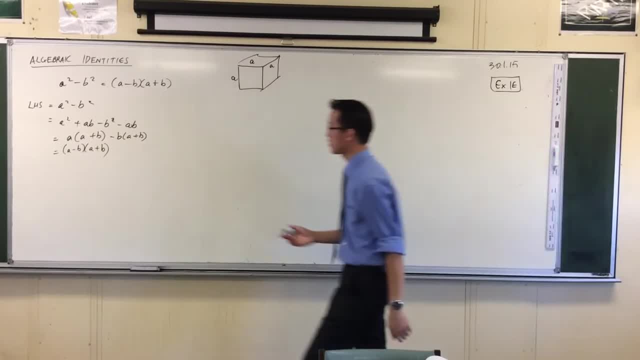 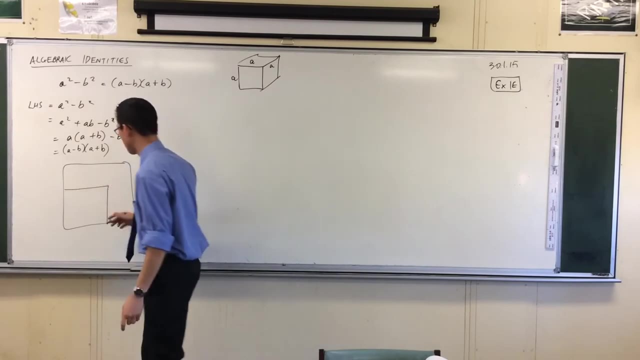 Okay. So if it's a square, if that's what it really means, if that's what this really means, what does this thing look like? It looks like a square minus another square. That's square-ish, right, Okay. 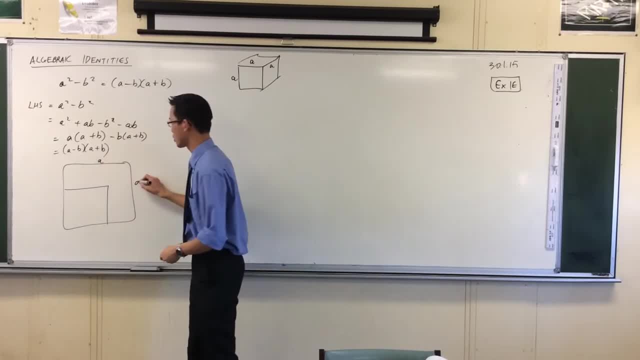 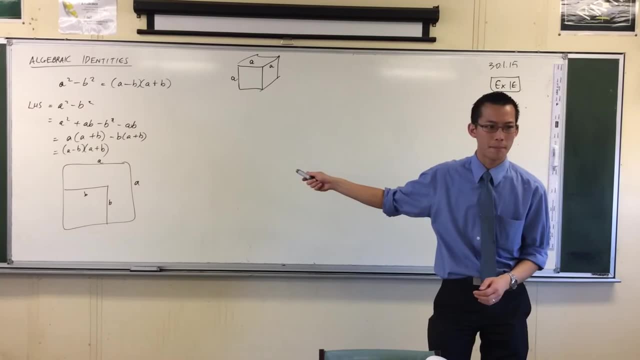 So A squared minus B squared. if I say this is A squared on the outside and this is B squared on the inside, where is A squared minus B squared on that diagram? Yeah, it's this. It's this corner part here, the L-shape. 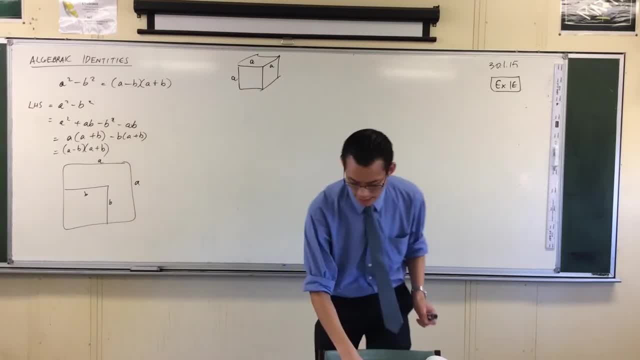 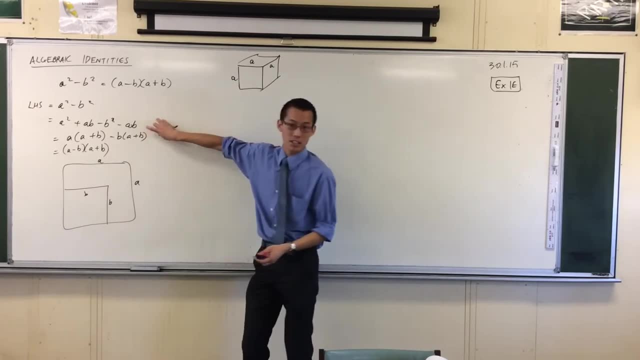 Rotated L-shape. Okay, So how shall I work out its area? It's not so hard, is it? There's lots of ways to do this, but a way that's parallel to what we did algebraically here with this suggestion is: 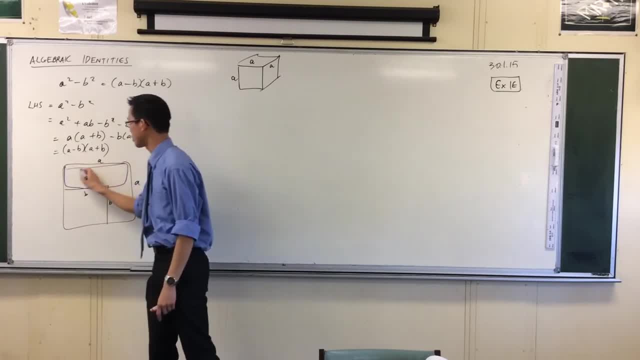 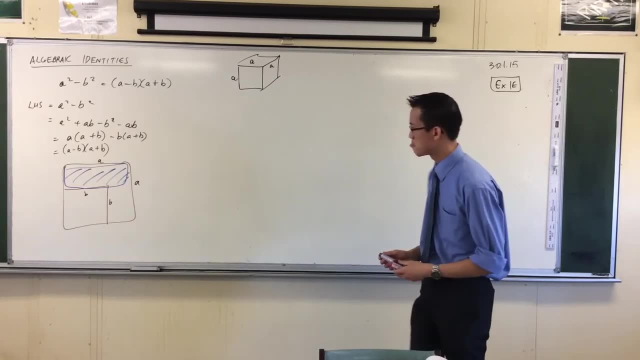 Well, just have a look at this part up here. Shader, Right That L-shape, it's a composite area. Tell me the area of the blue part: A times. Okay, It's A across that way, A times. 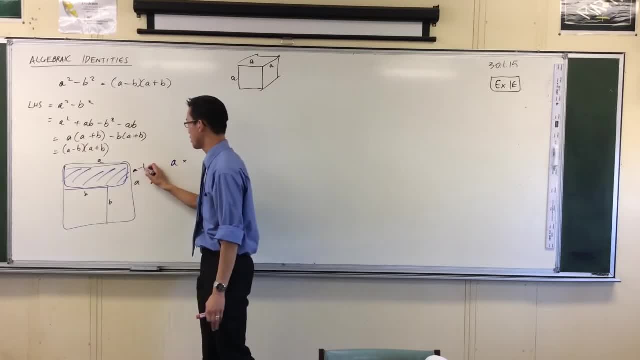 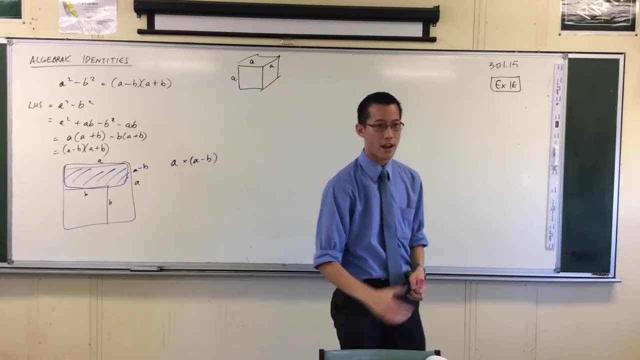 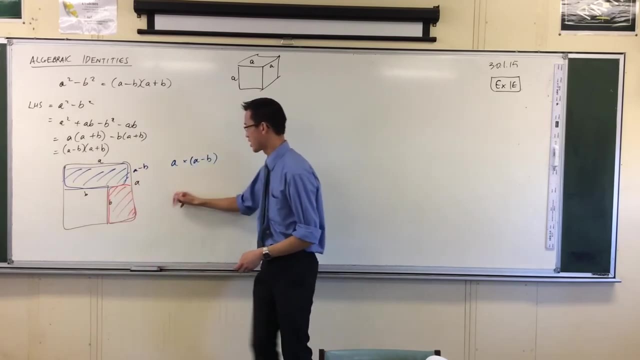 What's this? A minus B, A minus B. Good, Because Longer side minus shorter side. Okay, We have another area there, don't we? This guy down at the bottom? What's that? equal to B times, That's going to be B. 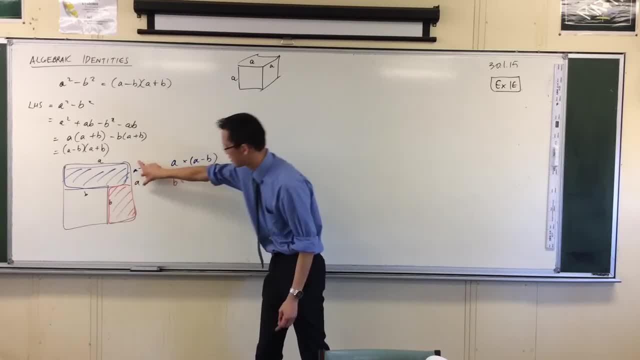 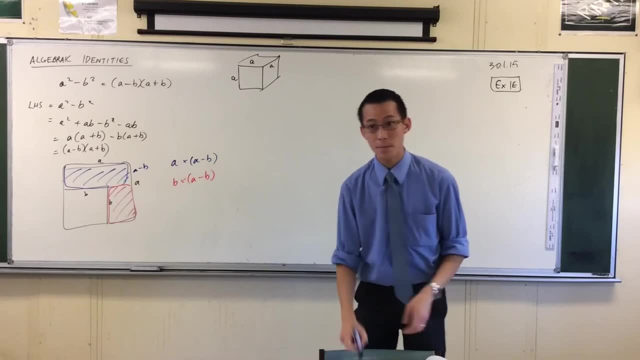 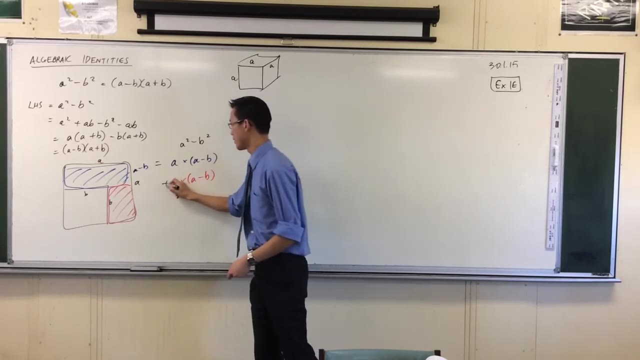 B Times: A minus B, A minus B. again, It's the same. There's a symmetry to it. It's a rotational symmetry. So there you go. That's A squared minus B squared. A squared minus B squared is equal to the blue plus the red, which looks to me similar. 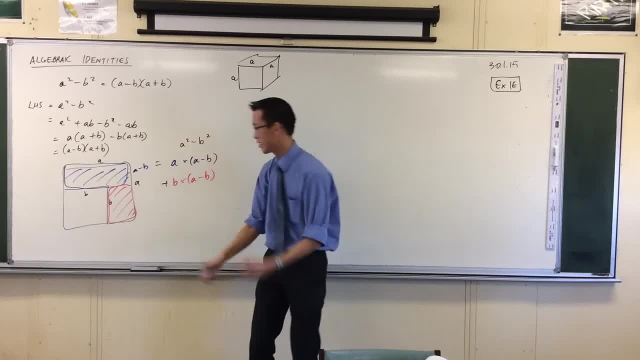 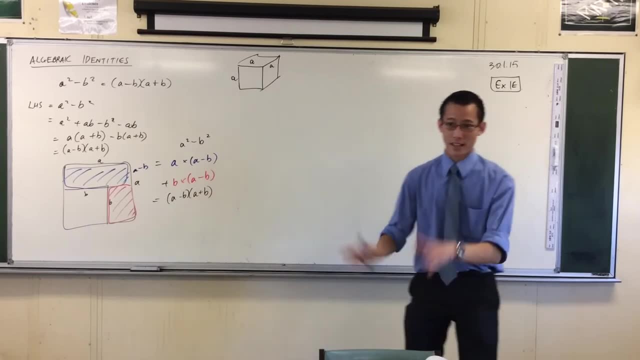 but not quite. You see how we factorized it. We've paired it the other way, But you're still going to get the same thing. Okay, All right. Familiar results: Some unfamiliar ways to get there. Difference of squares: that's a bit pedestrian. 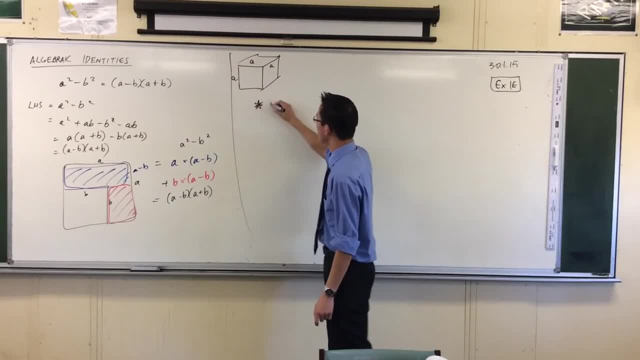 Let's move up to this guy. Difference of cubes. Okay, Now, the handy thing with the difference of cubes is that if you're trying to work out the difference here, that's one cubed minus another one, Okay, What's neat is that you can also do the sum. 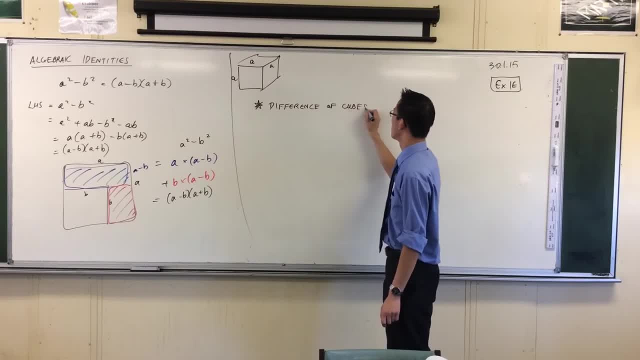 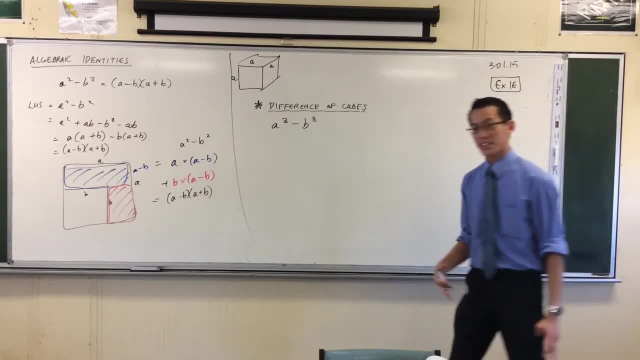 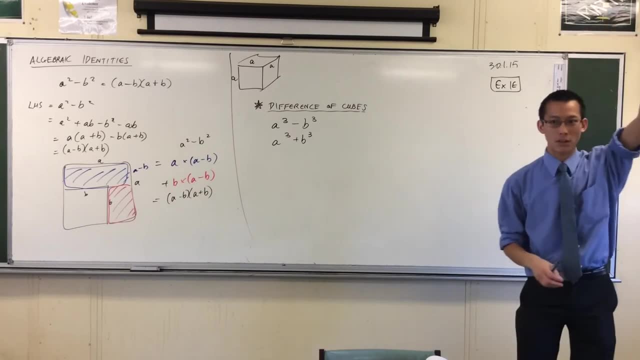 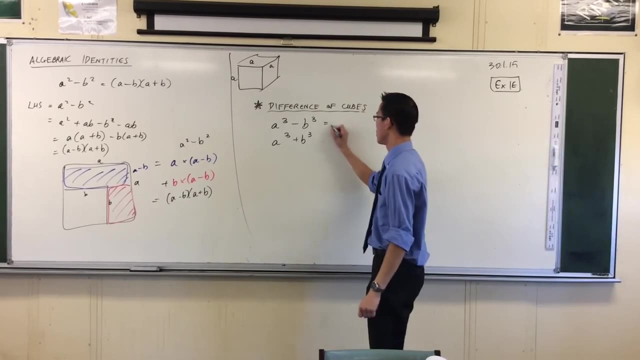 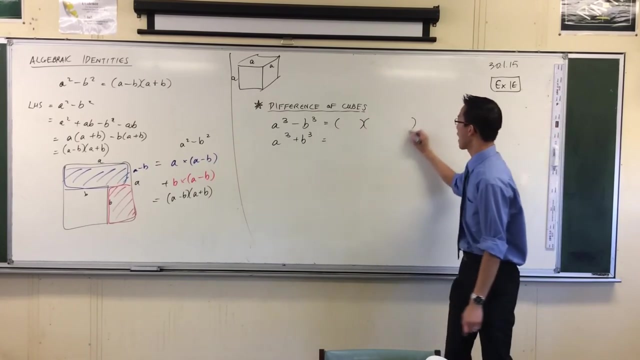 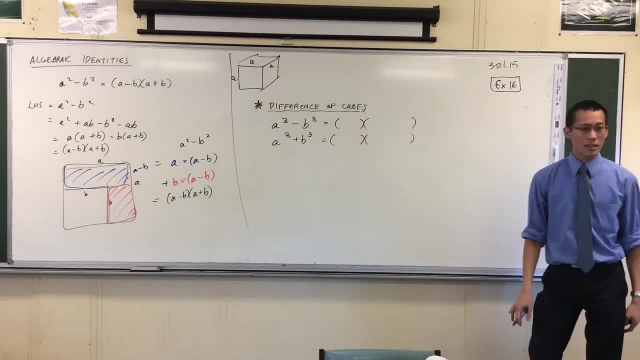 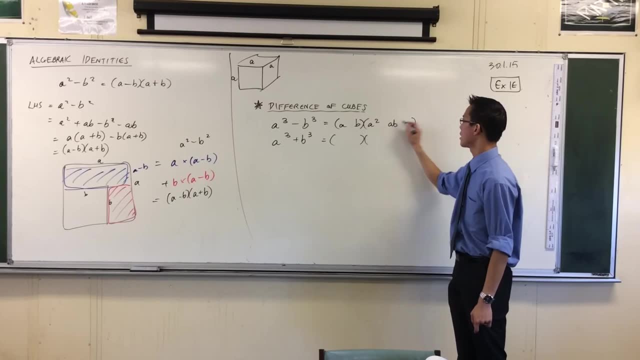 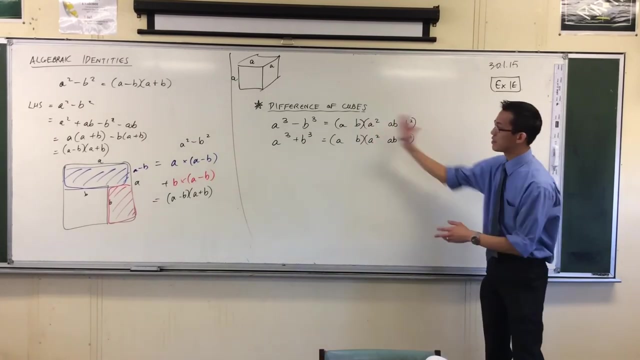 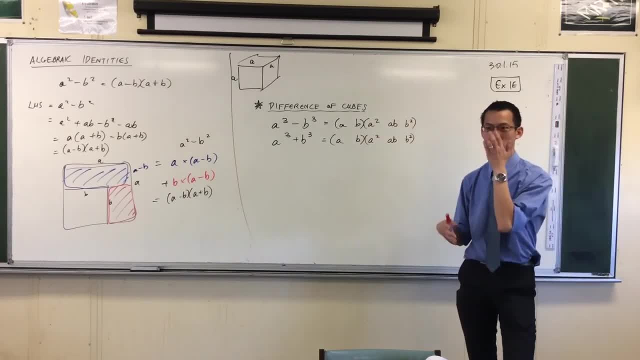 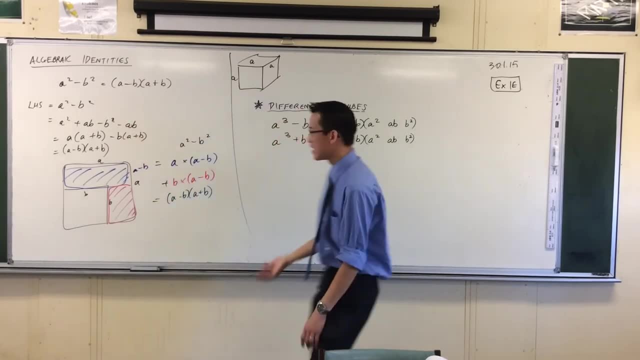 It's a whole series of pluses and minuses, And in a second I'm going to ask you to verify them by taking the suggestion you had in the beginning, which is just to look at that and then expand. It's sufficiently complicated that I won't make you do another way.